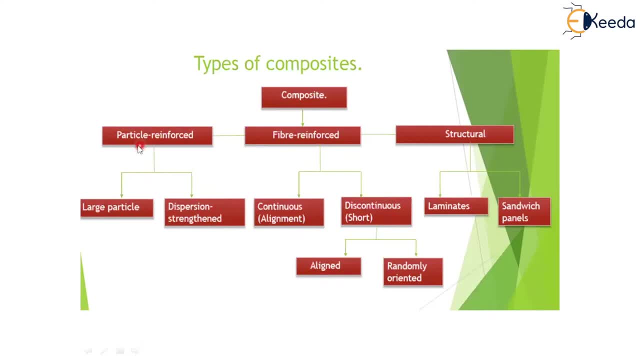 distributed in the material. So it depends on that the particle reinforced is again divided into dispersion strengthened composite material. The second category in composite material is fiber reinforced composite material. Fiber reinforced composite material means it is a. the shape of the reinforcement is in the form of fiber, like a thread. That means if you add a thread. 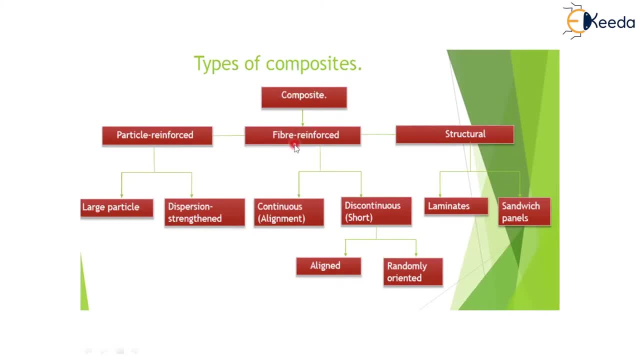 in the composite material that is like a thread. the second material has a thread. then the strength will increase. Compared to the particle reinforced composite material, it is also having a lot of strength and it is a vastly used fiber reinforced composite material In all the industries, not only in a single industry, that is, especially in structural world. 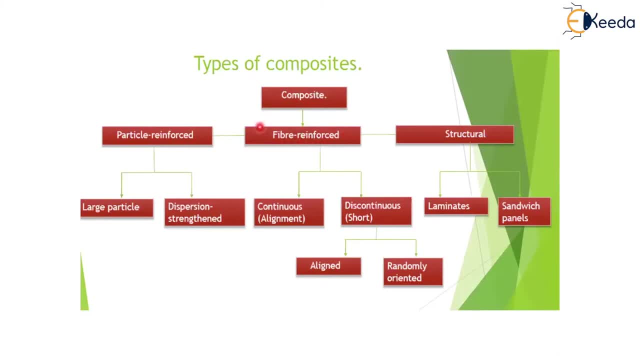 they are utilizing the fiber reinforced composite material. The best example is the concrete. Concrete is the best example for fiber reinforced composite material and we can see the second material. see, Sometimes we are adding the steel, The completed steel rods we are adding as a 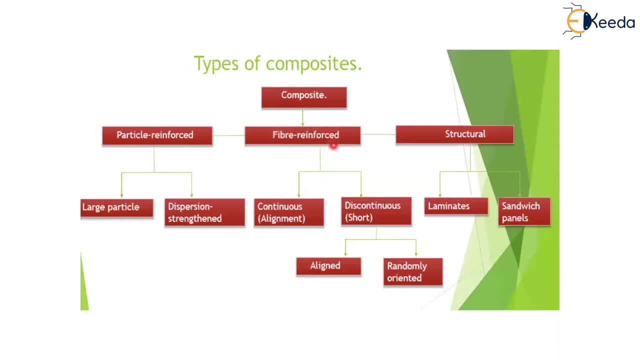 second, reinforcement in the pillars. So that is the one. Finally, I will give you a run at the metal, one type of composite, and stones are added as a mixture. there is a reinforcement in the concrete that is called as a particulate reinforced composite material. now let me explain the fiber. 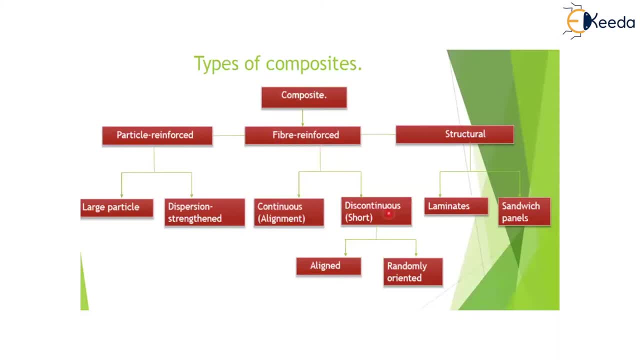 imposed. composite material is divided into continuous and discontinuous. continuous and discontinuous means if the fiber is a continuous, that means a long thread is used as a reinforcement so that can be represented as a continuous reinforcement. continuous fiber- reinforced composite material. if it is a discontinuous, that means if the short fibers are used. 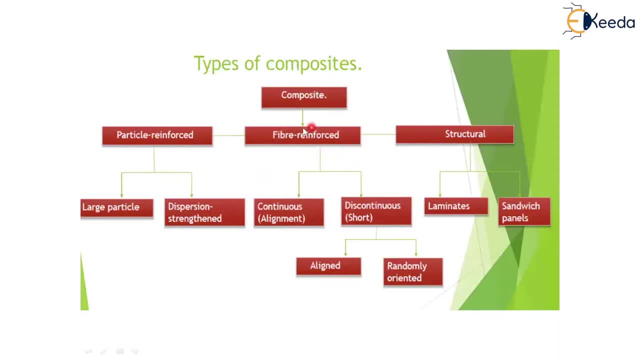 then that type of composite material is represented as a fiber reinforced. that is, a discontinuous fiber reinforced composite material. anyway, it is again classified. that is depends on whether it is a aligned or randomly oriented, depending on the requirements. Sometimes it depends on the customer's required properties. 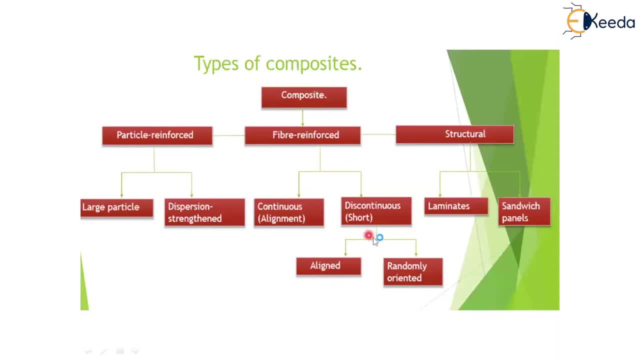 We can go for the aligned short fibers or randomly oriented short fibers. It completely depends on the requirement. Now, the third category in composite material is structural composites. The structural composites, or the laminar composite materials, are divided into laminates. That is here the laminates. that means, layer by layer, we are adding the material and we are forming as a composite material. 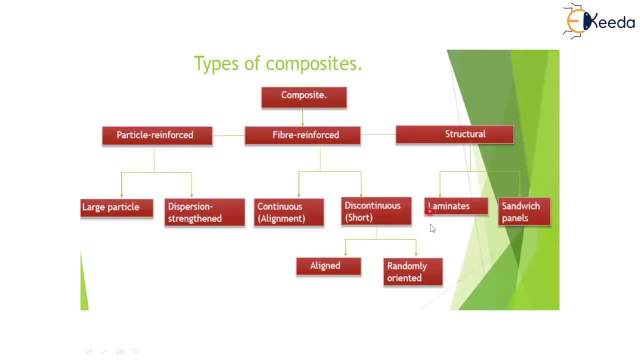 One layer is made with a different material, Another layer is made with a different material. So these type of layers depends on the requirement. We can go for the structural composite material, The next one, the same structural composite, that is a laminar composite material, is again divided into sandwich panel. 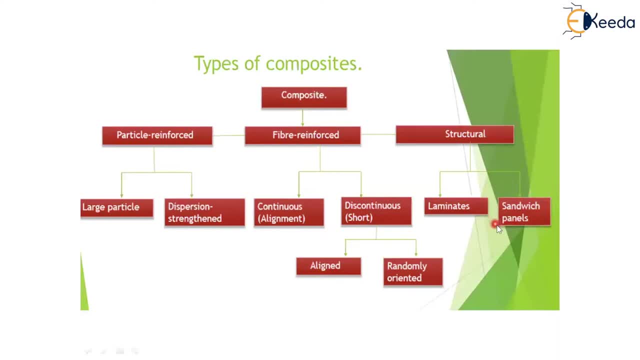 Sandwich panel means two. Two layers are of same size And in between that another reinforcement is available, That is, it represents a sandwich panel composite material. So these are the three classifications. There is a particulate reinforced composite material, fiber reinforced composite material and structural composite material. 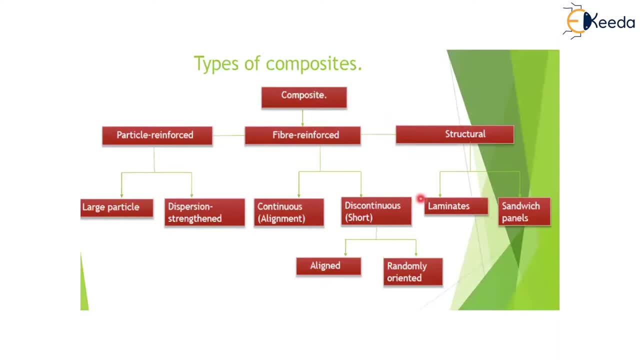 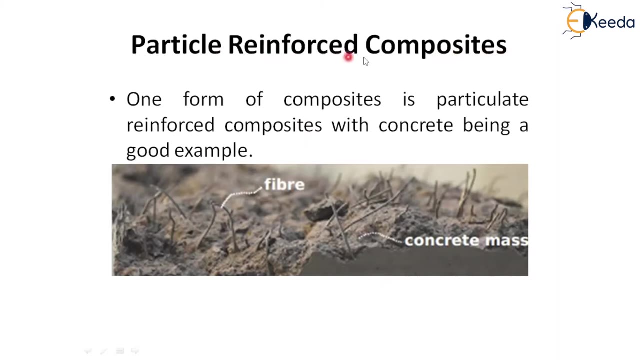 So these are the three in general basic composite material types with which we can make the materials in different. We do not use single blocking and it depends onitchen. The design of the material has to groupe from these three components, So we will use volont suspects. 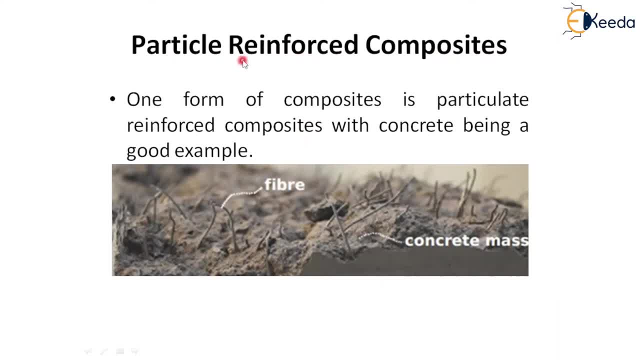 And this component. we have to separate it爾го and 엄το. These components are built at the right long distance. Now they must be placed at the right length And since they are дальше than forward, we need to separate them from theirродunivers. 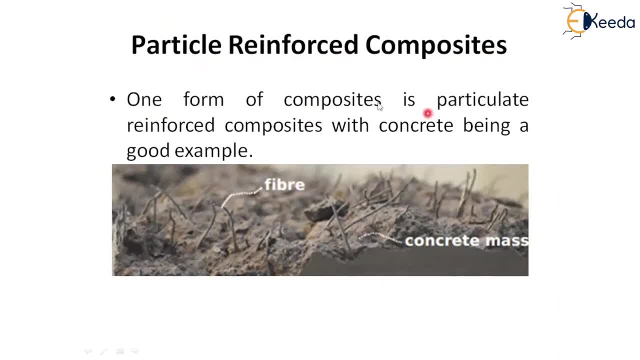 So it's more this, of course, and therefore We have a contribution. And these groups are all based on the same components in parallel, And then there are two components. these as theっ concrete is, it being a good example here ivory has also shown, and in the same concrete we can. 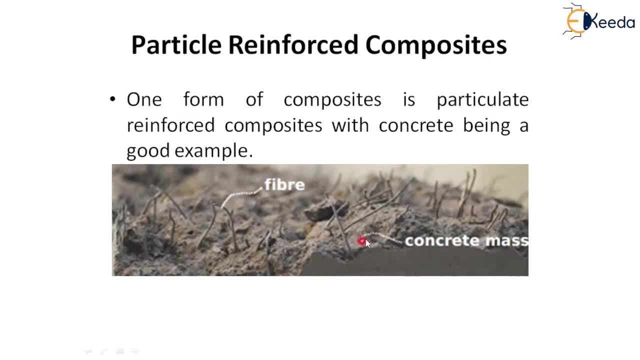 see the particles here, the concrete mass. so these particles, a lot of stones are available here. these stones are represented as a particles which are added in the concrete. so the same concrete can be taken as an example for the particulate reinforced composite material, as well as fiber reinforced composite materials. that means, if you take these tools as a second reinforcement, 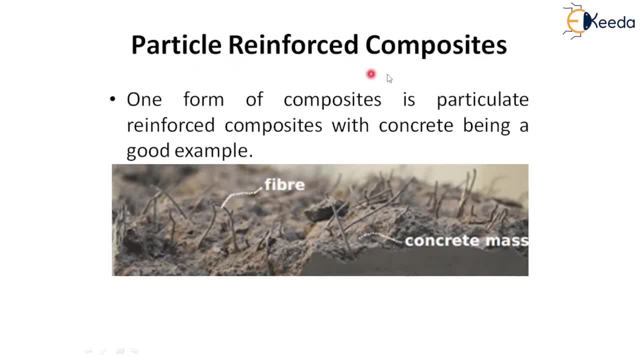 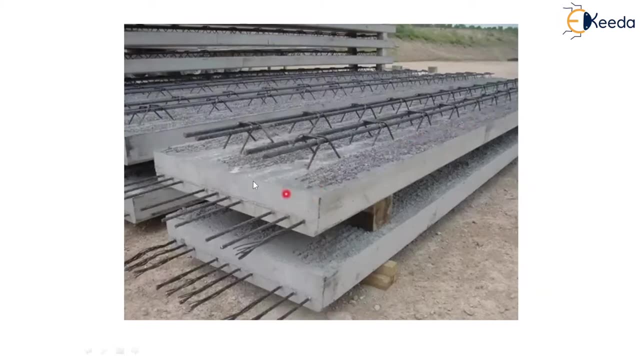 then we can say that composite as a particulate reinforced composite. if you take the fiber as a reinforcement, that is, as a second material, then we can say that composite as a fiber reinforced composite material. you can see, here is a concrete product and in this the steel rods are placed. 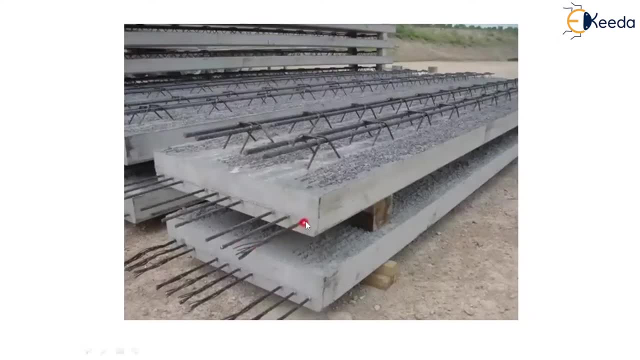 so this is- we can say that it is- a continuous fiber reinforced composite material and at the same time, some stones are mixed to manufacture that produce this particular concrete. so this is also an example for the particulate reinforced composite material and you can see this: all the rods are available and it is. 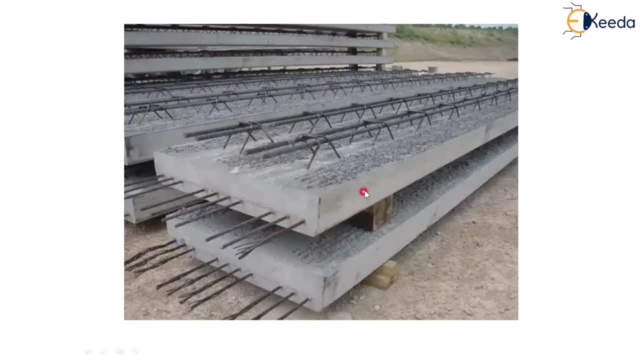 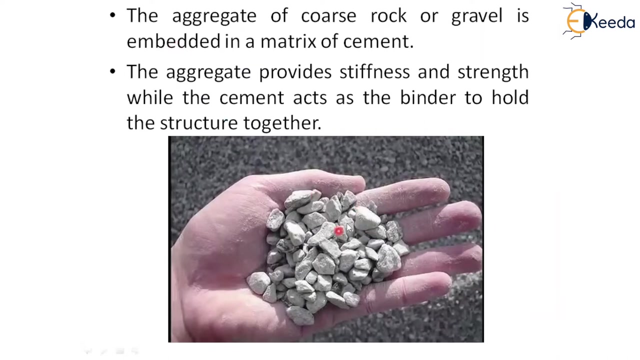 induced in the concrete mixture. that means the total load. whatever the load given to it is taken by the these fibers, that is, steel rods, they will act as a reinforcement, it will increase the strength. so this is a fiber reinforced composite material and it is also an example of, particularly if you see the strange stones. so these aggregate of 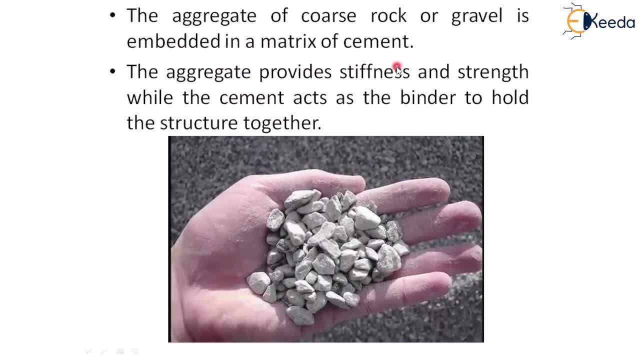 coarse rock or gravel is embedded in the matrix here. so that means this aggregate provides the stiffness, whatever stiffness that you want. you can get the stiffness and the strength, while the cement binder to hold the structure together. so to hold the structure one must be act as a binder here. 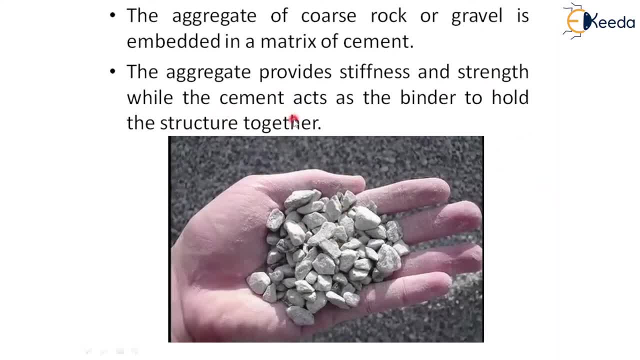 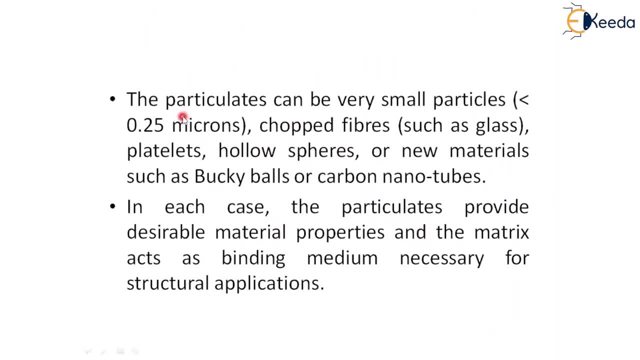 suppose if you take this type of quarter the cement acts as a binder to hold the structure that is in the structures it will hold as a binder. and especially if you see the various features of the particulate reinforced composite material, the particles can be very small particles maybe. 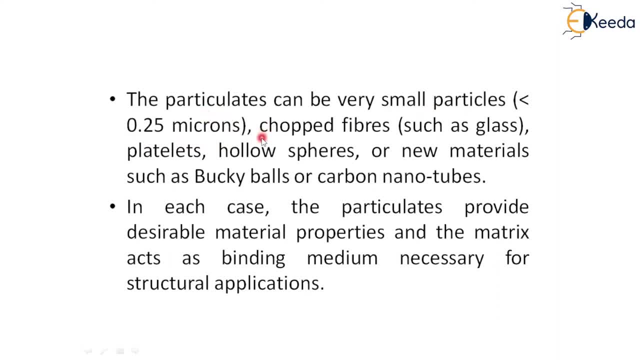 sometimes it is less than 0.25 microns. and chocolate piper suppose glass pellets, hollow spheres or new materials such as bulky balls or carbon. so so many examples are available. in each case, if you take any case here, the particulates provide the desirable material. 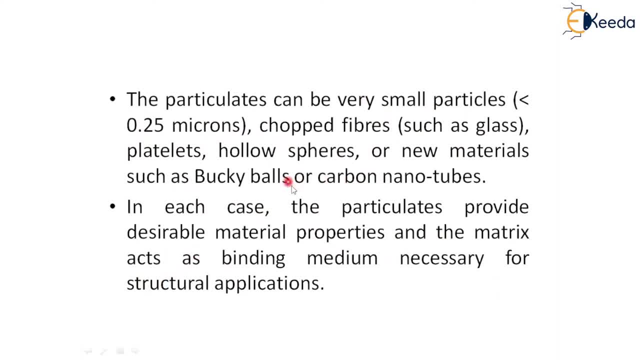 properties and the matrix, whatever the matter that you have taken, act as a binding media. so that means all the particles has to stick together and has to give the strength to the material, whatever the necessary for the structural applications. what are the necessary strength required by the material these reinforcement will give? so this is a particulate reinforced. the next one is a fiber. 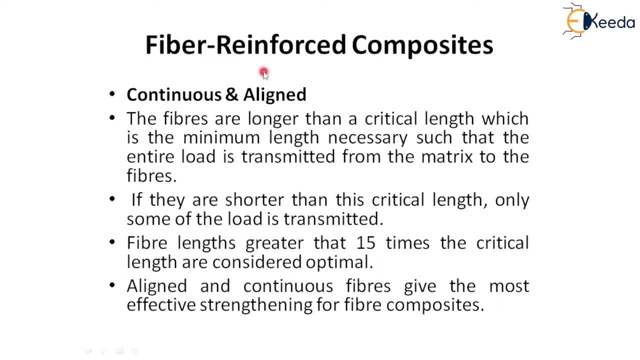 rainfall, as we have seen the concrete shape in that the steel rods are aligned. here. that means if you add the second material as a fiber, that means in the form of the thread, so then that type of composites are represented as a fiber. reinforced composite material, material. sometimes it is a continuous, that means the fiber may be continuous, so sometimes it is. 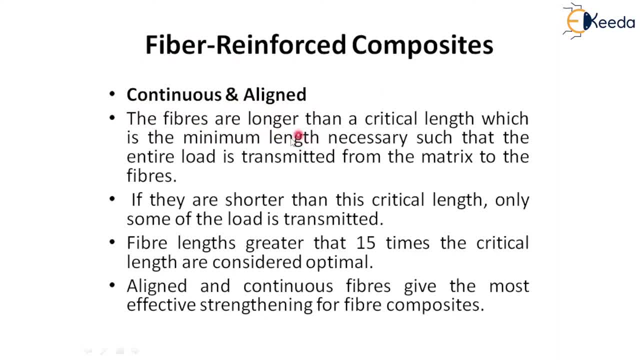 aligned. see the fibers. whatever the fibers that you have taken, no longer there is a longer than the critical length. the particular means which is a minimum length necessary to have the load, the entire load. if it is on the material, it has to bear it. so how much length is required? 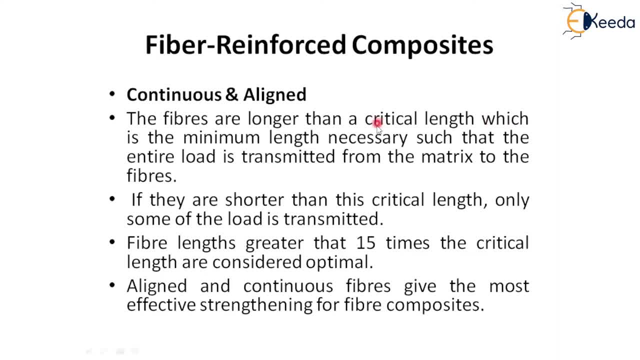 so that length you have to represent as a critical length here. so that means, if they are, suppose, if you have calculated critical length for a particular material. and anyway, one thing i want to say. the critical length varies from material to material. if they are started in the critical length, only some of the load is transformed. that means what? 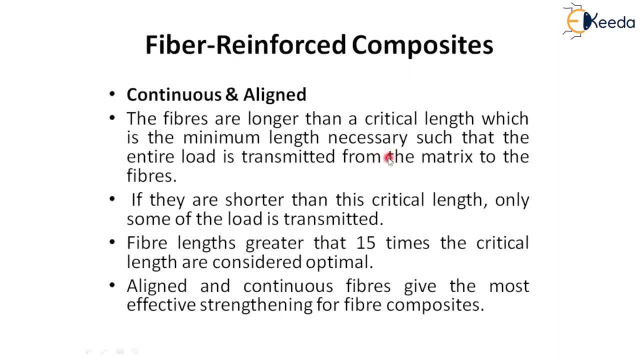 are the material that you have taken, if you want to add as a reinforcement. so it must be matched to the critical length. if it is shorter it will be no longer works for its purpose and in general the length of the fiber is almost greater than it is a 15 times the critical length. 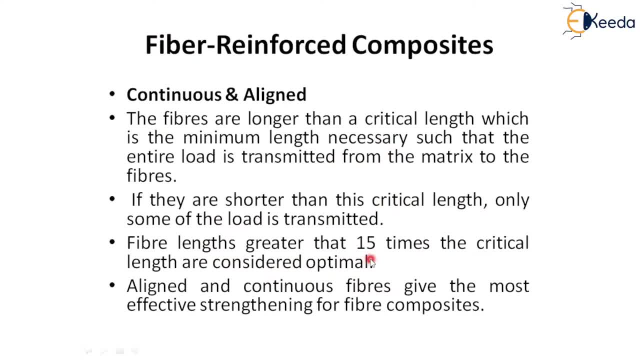 so consider as a optimal. so then it will bear the total load. see, the condition is in the critical length, the length we are not supposed to take, the less length than the critical length. but you can take the maximum length that is more than the critical length. that is accepted and that is. 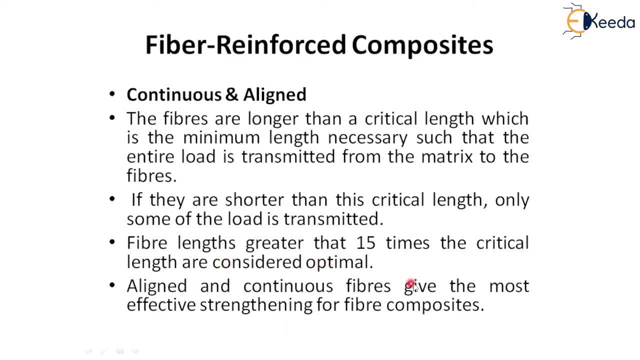 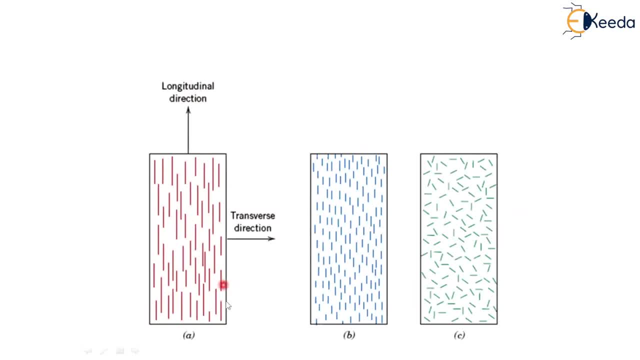 allowable length and what are the alignment continuous fibers and give the most effective fiber composites. you can see the difference here. this is in a longitudinal direction. this is the perpendicular to longitudinal or perpendicular to the material is a transverse direction. all the fibers are arranged like this. you can see here. here also all the fibers are. 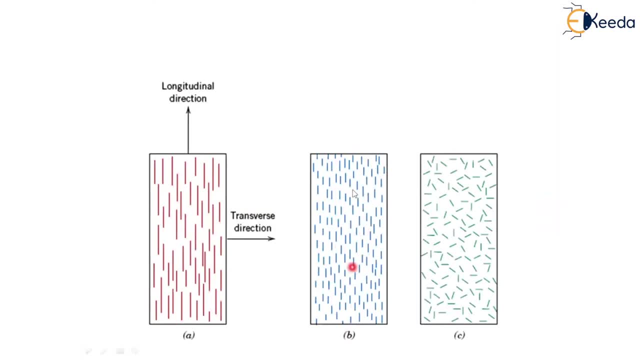 arranged. but compared to this this is a shorter fiber, short fibers, and here they are not aligned. see when. depends on the requirement, depends on the properties required. you can go for the continuous fiber, reinforced composite material or discontinuous. it is almost not aligned composite materials, so both can be used for different purposes. both are based already. 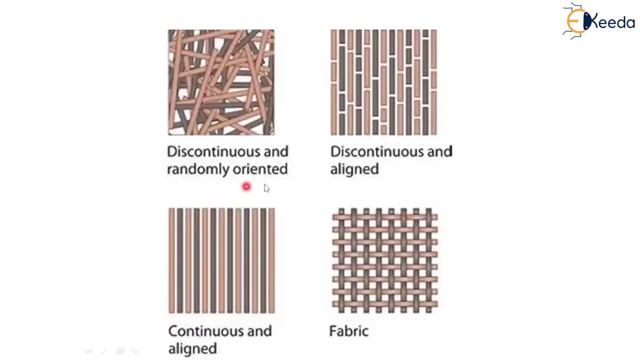 they are available in the market. now you can see in another manner: this is a discontinuous and randomly oriented. this is discontinuous and aligned and this is a continuous and aligned. that means longer reinforcement. there is a longer thread is available here. this is a fabric. this is the best example how it is useful for the reinforcement, how the reinforcement 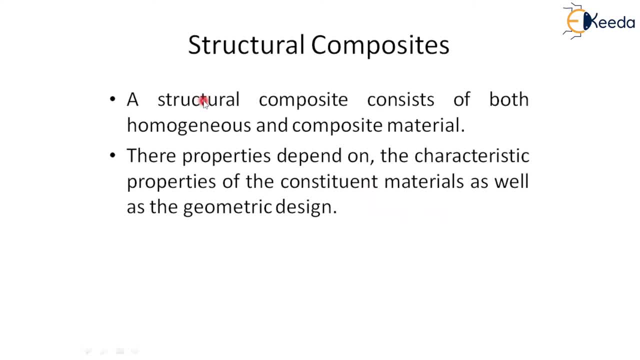 is useful. and the next one is the third type is structural composites. structural means it is by layer, by layer. in general, what are the structural composites that you have taken? the both homogeneous. that means whatever layers that you are going to take, that must be homogeneous. 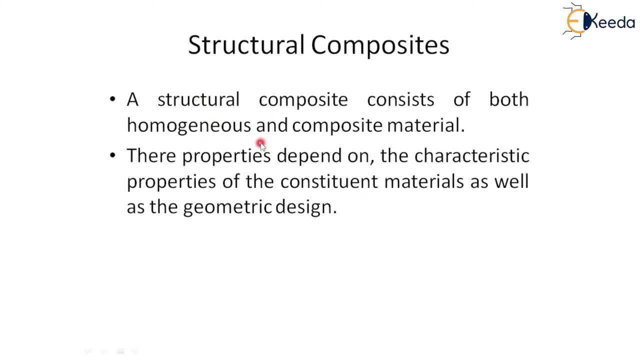 that means almost of the similar type of properties and of the same nature. these properties, what are the properties that you have taken? and after that, if you calculate, that completely depends on the characteristic and the constituent materials, as well as the geometric design. so that means, if you want to maintain a homogeneous material, all the sandwich. 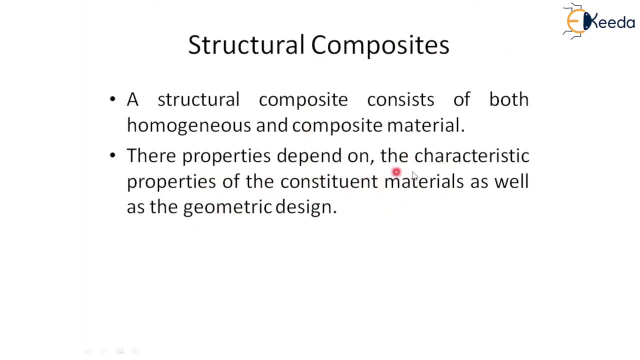 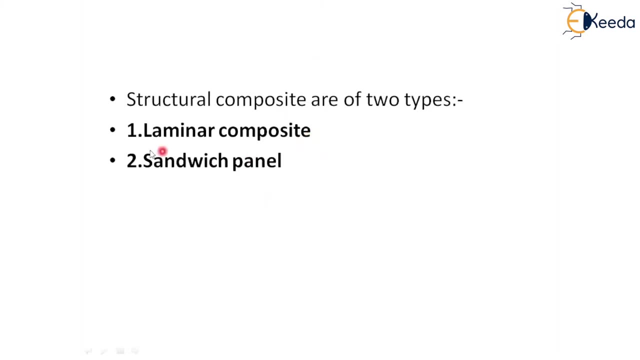 material or all the layer. the materials must have the different properties and all must have the same properties and the characteristic properties of the constitutivity. we have to check all these properties to have the layer and then we can see that the material is not a composite material, that is a structural composite. 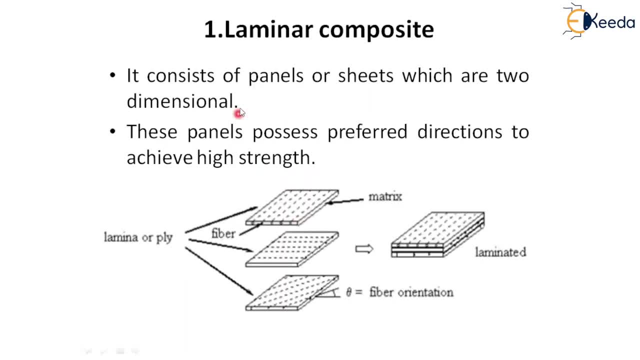 material. you can see the two types are here. one is a laminar composite and one is a sandwich panel. if you see, the laminar composite material you can generate consists of the panels like this sheets, which are in general two dimension. these panel actually possess a proper direction to achieve. 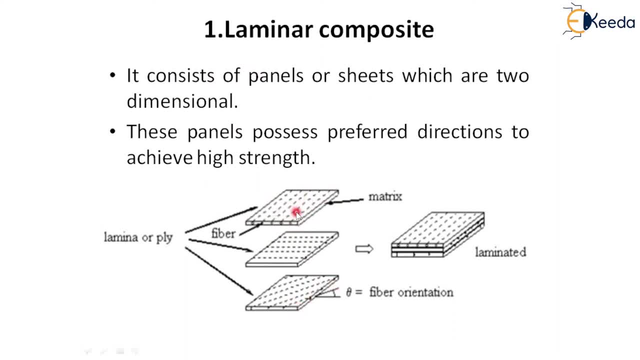 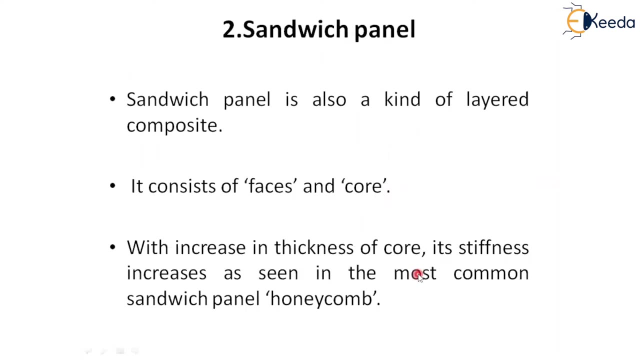 the high strength you can see. here you can see all the directions are aligned. so by keeping this type of arrangement you can make laminar composite material or, if you want, if both sheets are of same material in between. if some other material is available, then we can say that it is a sandwich material, sandwich in general. 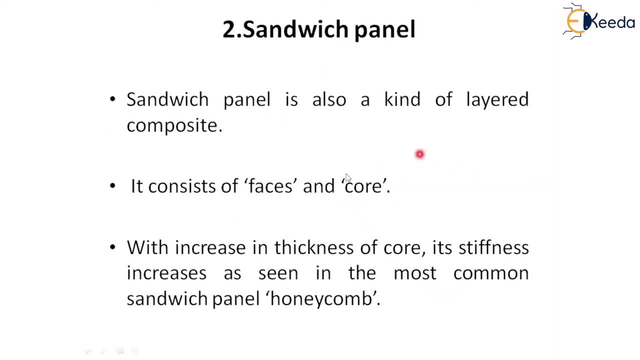 just now we have seen the sandwich material: two layers of same shape. the middle one is of another shape and another material. so in general it consists of faces and core. whenever the suppose the thickness of the core, it increase the thickness of the core generally, its stiffness also increase. 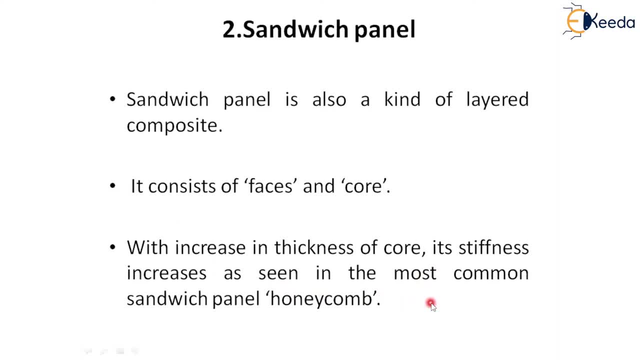 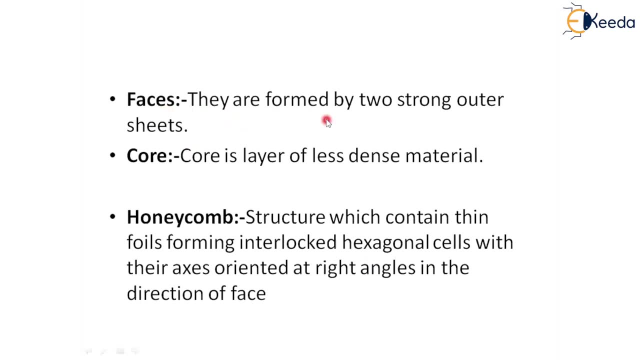 in the most common cases, that is especially honeycomb sandwich. i will show you how the honeycomb sandwich looks like and the faces here. in general they are common with the two strong outer sheets, and core is always less than the dense material. so let us see the honeycomb structure between two. 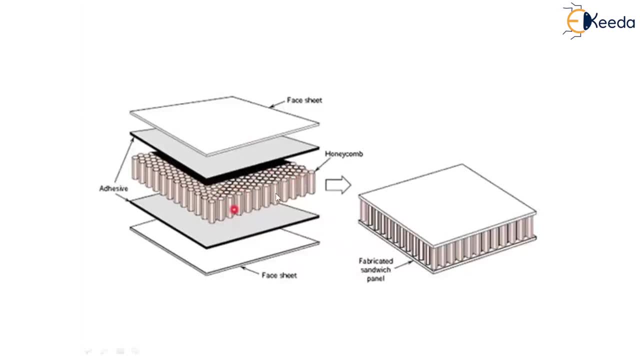 layers. so this type of structure will give the maximum advantage compared to any other material. so these are the face sheet, this is the bottom sheet and other material is the outer material. so a layer by layer. some other sheets has came, so this is a laminar composite material. this is like. 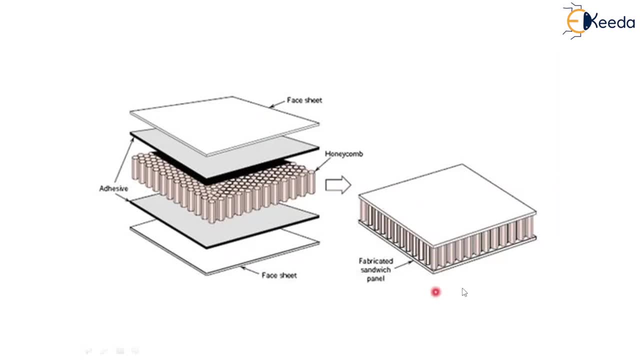 a fabricated sandwich panel. so the top one and the bottom one are of same material, but the middle one is up with us different materials. if this is the arrangement, then we can say that it is a sandwich type of composite material. so this is all about the various composite material. that is the 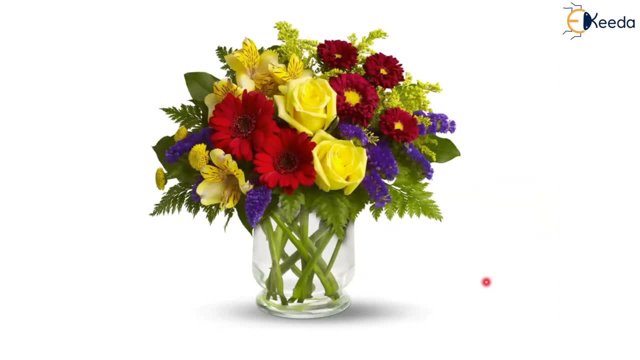 types of composites. in the next sessions we will discuss some of the technological points and in material technology. so this is all for today, thank you. thank you one another.